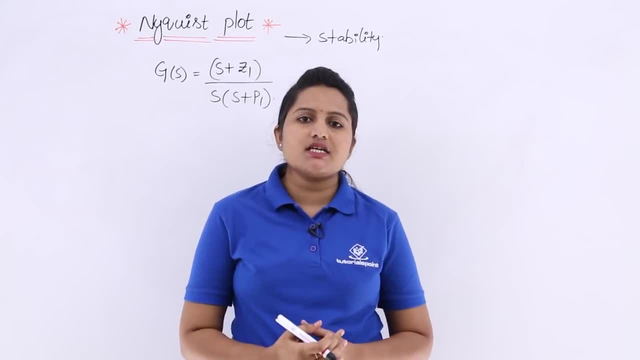 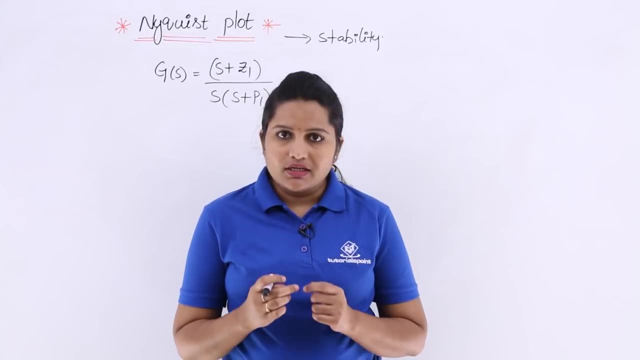 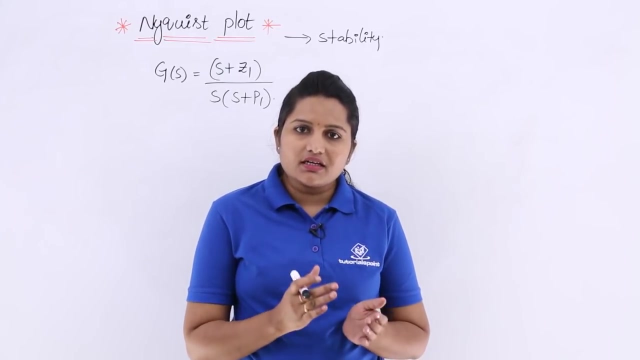 In this video we are going to discuss stability of Nyquist plot. As I already told you, polar plots are similar to Nyquist plots, So the Nyquist plots are just extension to polar plots. So here in polar plots we are going to consider the transfer function from: omega is equivalent to: 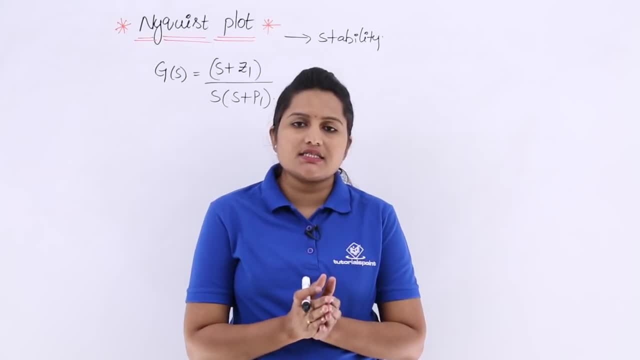 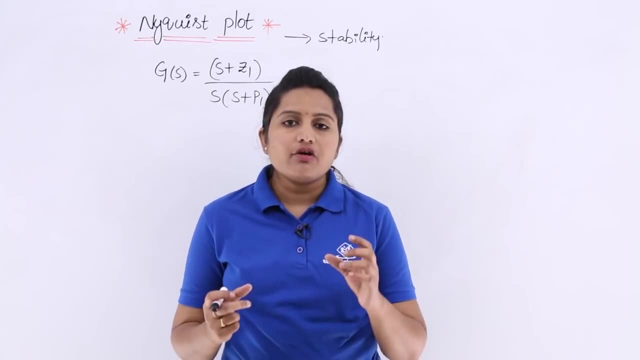 0 to infinity. That means we are plotting from. omega is equivalent to 0 to infinity, Whereas in Nyquist plot, as that is extension to polar plot, we are going to plot that plot from minus infinity to infinity. So we are going to extend that open loop transfer functions plot from minus. 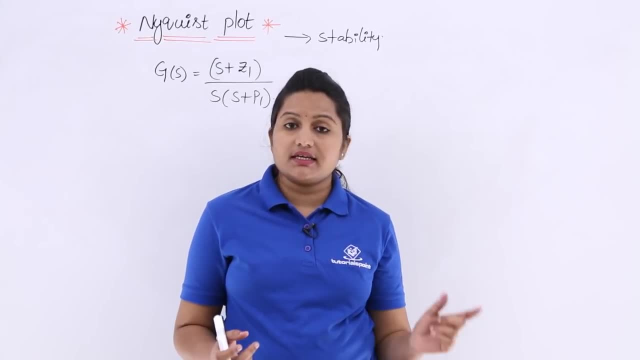 infinity to infinity, Whereas in polar plot case we are taking from omega is equivalent to 0 to infinity. So we are going to extend that open loop transfer functions plot from minus infinity to infinity, Whereas in polar plot case we are taking from omega is equivalent to 0 to. 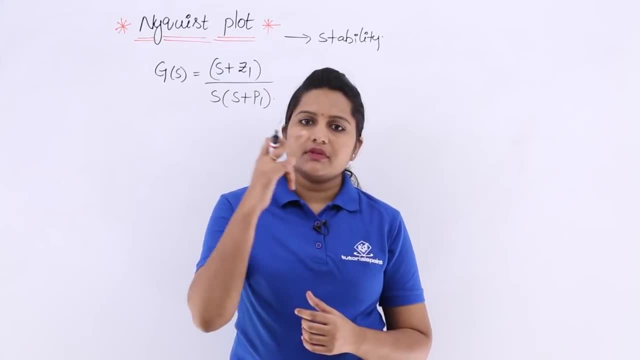 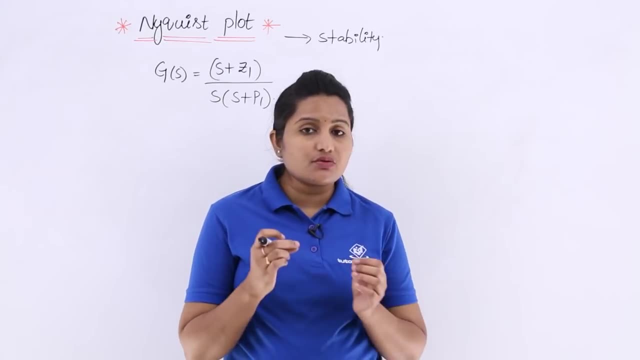 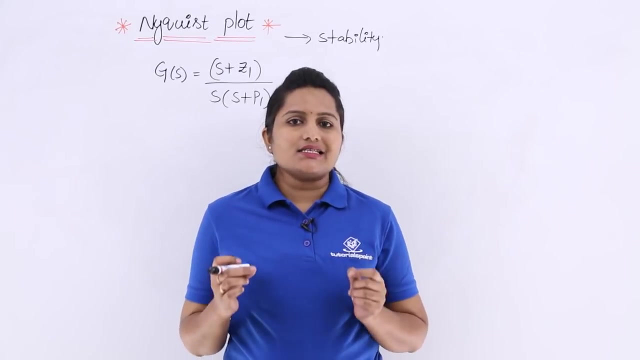 infinity. So here we are observing the magnitude and phase of a open loop transfer function from minus infinity to infinity. This is only the difference. remaining is same as polar plot. So in initial classes of polar plot, as I told you, polar plot is same as Nyquist plot. 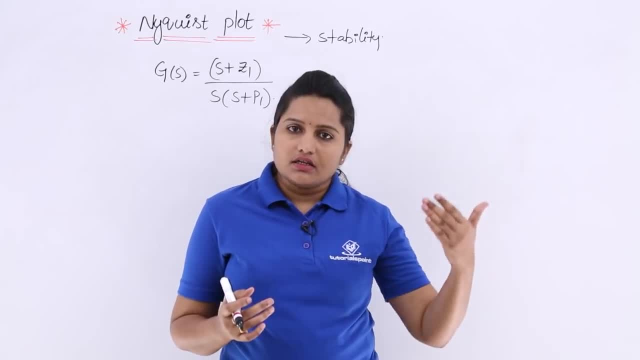 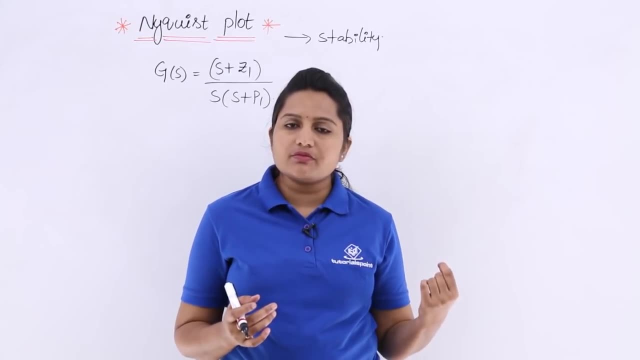 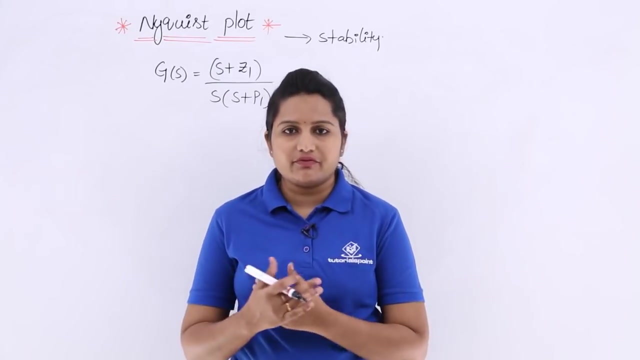 but the single difference is there. we are taking plot of magnitude and phase from the values of omega, from 0 to infinity, Whereas here in Nyquist plot we are taking the plot from minus infinity to infinity. Now, when you are examining about the 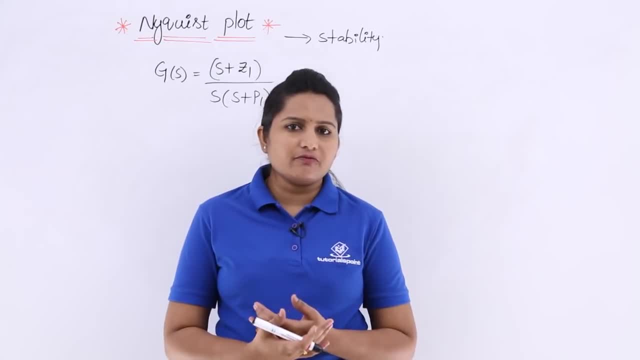 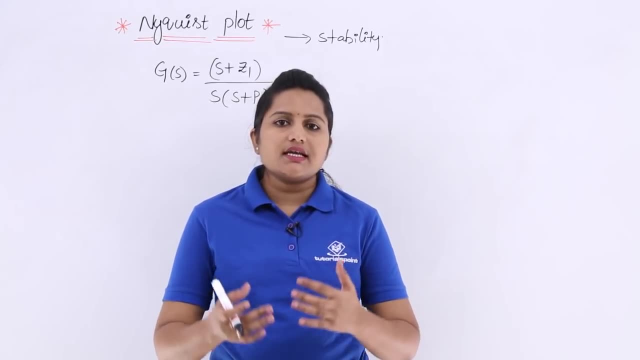 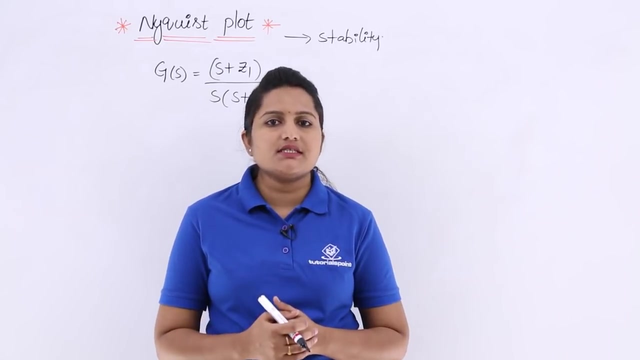 stability. all these plots are for stability analysis. So to examine the stability, how a system is said to be stable When a Nyquist to polar plot is said to be stable, the Nyquist plot is said to be of stable system, Nyquist plot. So here we will see about that. 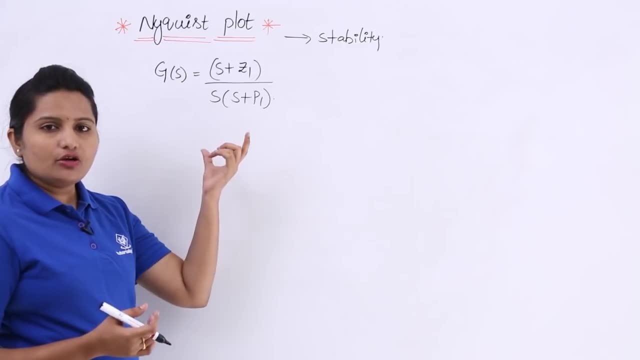 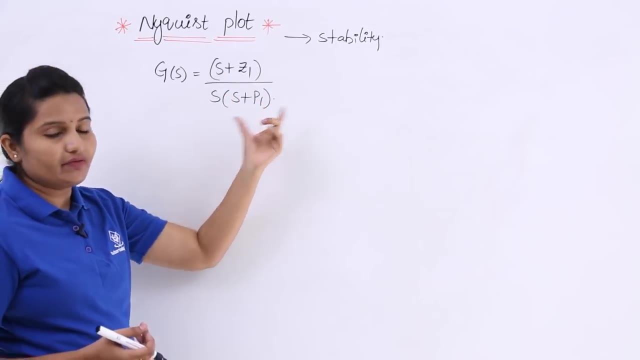 So now, here this is the open loop transfer function of the system. This is: g of s is equivalent to s plus z1 by s, by s plus p1.. So here I am having two poles: one pole at origin, one pole at some other places is equivalent to minus p1 pole, And here s plus z1, I am having 1: 0. 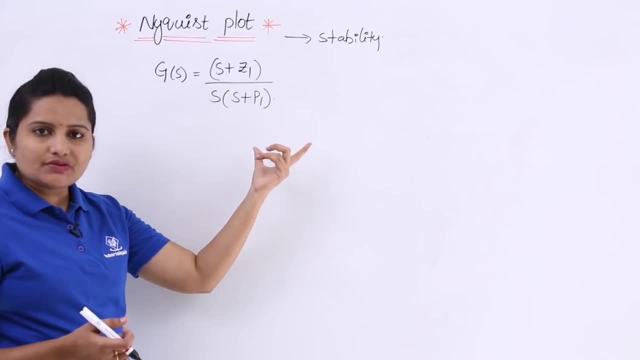 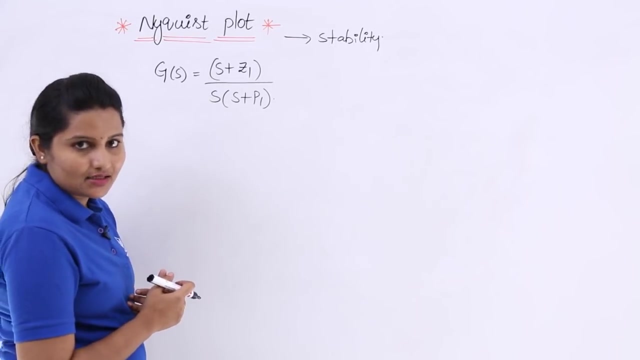 The numerator of this transfer function indicate zeros and the denominator indicates poles. So now here I am going to examine the closed loop transfer function to get the stability analysis. That means c of s by r of s. this is closed loop transfer. 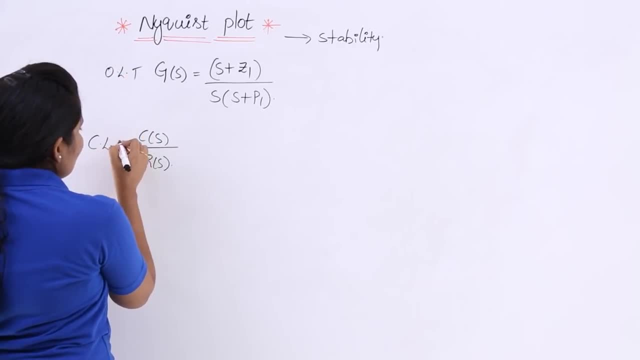 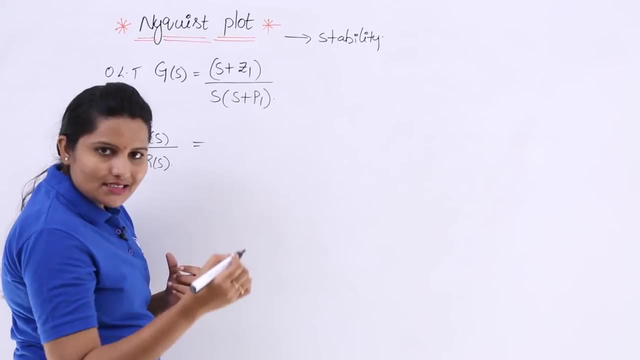 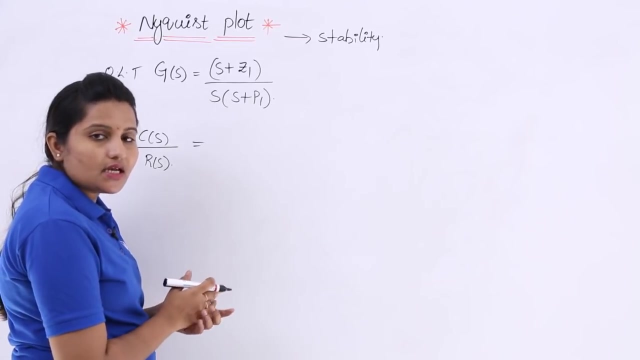 function. This is open loop transfer function. this is closed loop transfer function. c of s by r of s. How we will get this? So this is: as this is negative feedback system, For example. I am considering negative feedback system Whenever I discuss this. feedbacks, as I told you. 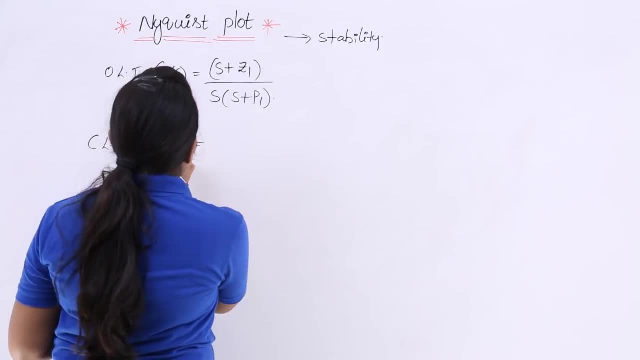 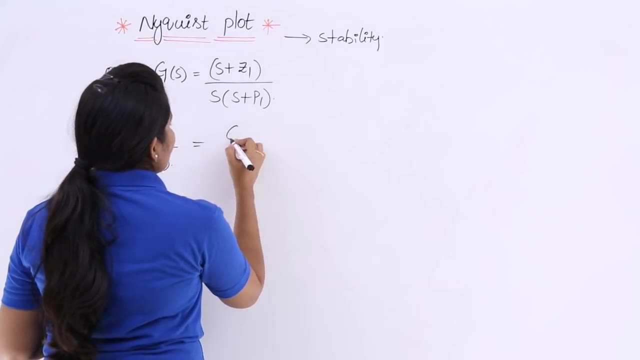 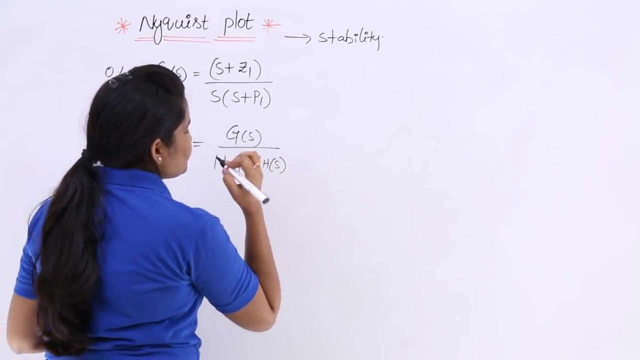 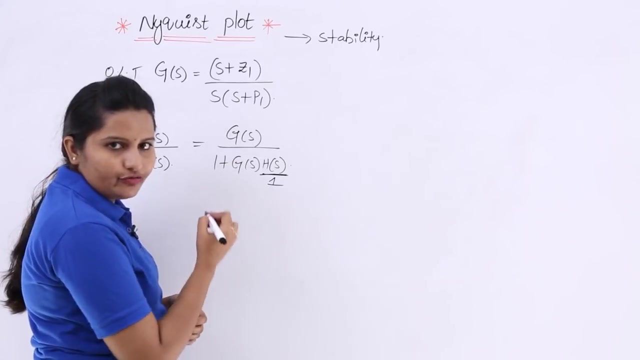 negative feedback is preferred in control system. So here the negative feedback control systems transfer function. closed loop transfer function is equivalent to g of s by 1 plus g of s into h of s, Where h of s is equivalent to unity for unit negative feedback system, That means h of. 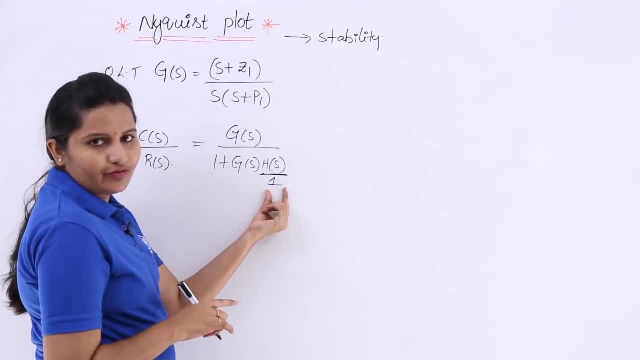 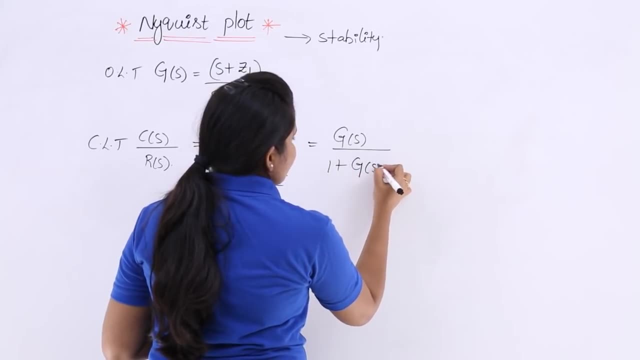 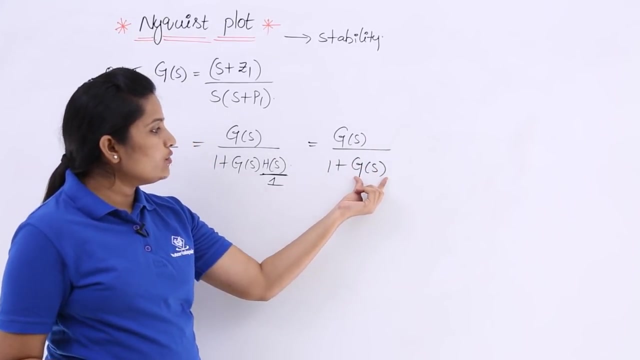 s is equivalent to 1 for unity negative feedback system. So this is equivalent to g of s by 1 plus g of s. Now you can see g of s by 1 plus g of s. So here you know about g of s you already given. 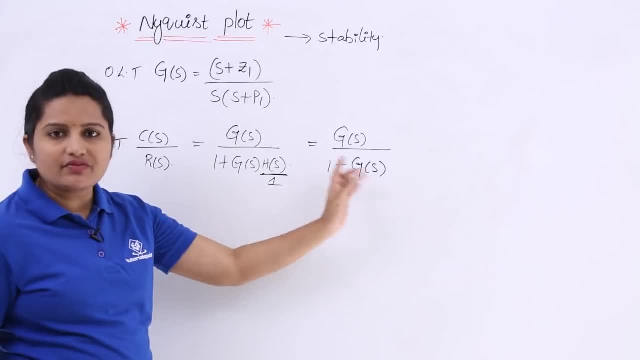 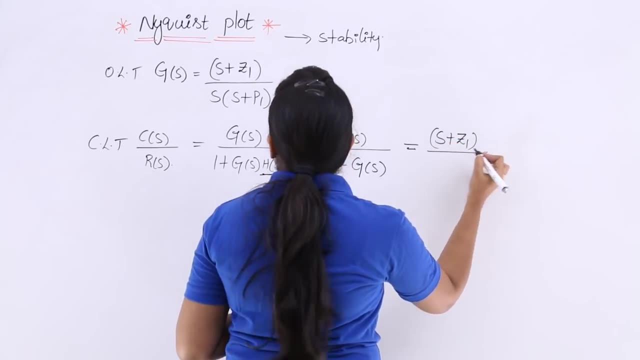 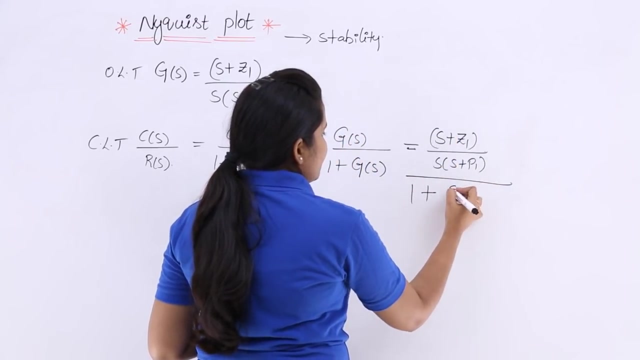 with g of s. So I am going to substitute that g of s value here. So now this is equivalent to s plus z1 divided by s into s plus p1. divided by this is g of s 1 plus. again I am repeating this. 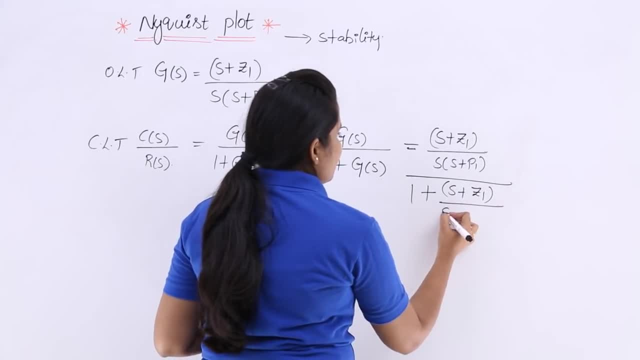 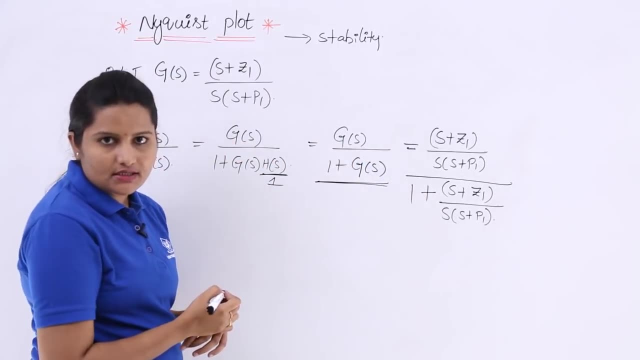 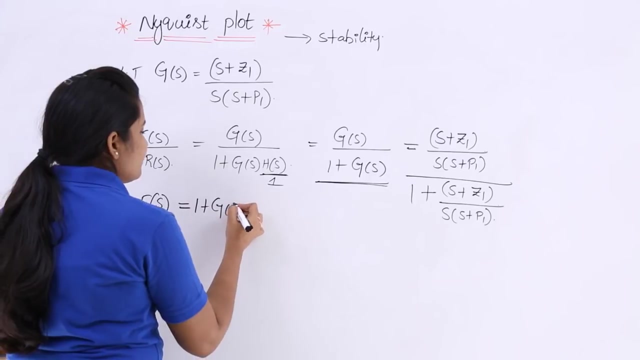 g of s, So s plus z1 divided by s into s plus p1.. I am considering this denominator as f of s. So here I am considering f of s is equivalent to 1 plus g of s. So 1 plus g of s means this one. 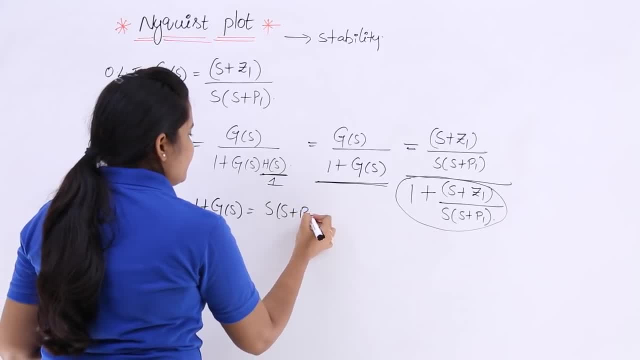 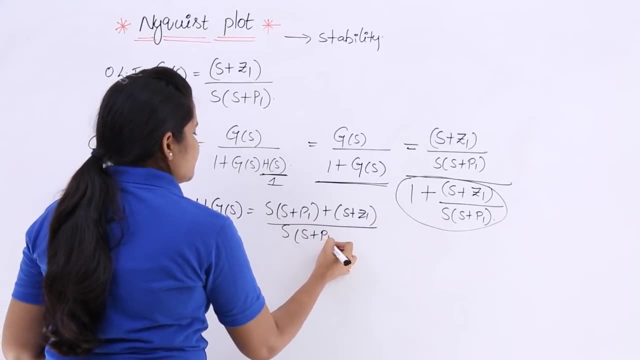 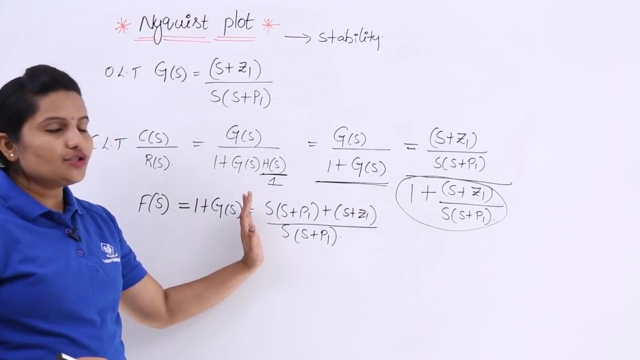 So I am cross multiplying s into s plus p1, plus s plus z1, divided by s into s plus p1.. This is what we are going to get. So 1 plus g of s into h of s. I am considering like f of s. 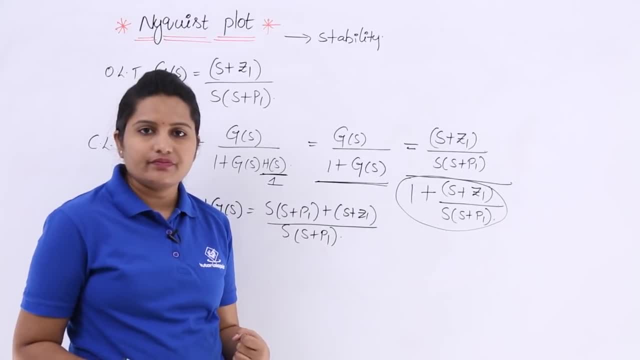 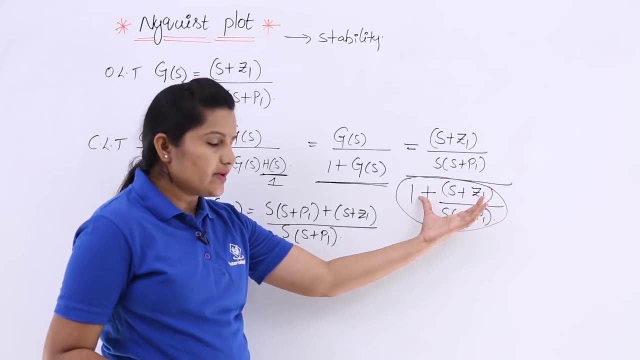 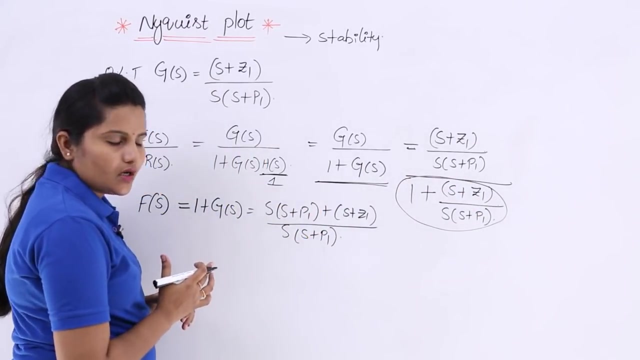 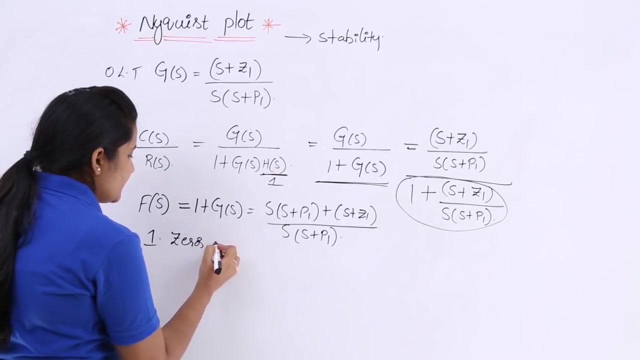 So that f of s will be like this. So now here, if you observe, if this is f of s, if this is f of s, So if you observe, you just imagine this term here. So the zeros, first point you need to understand is the zeros of f of s are poles of. 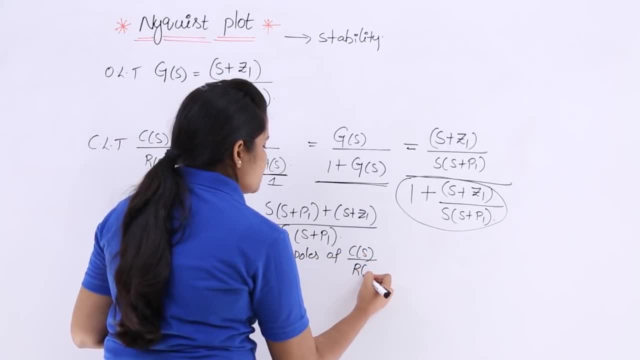 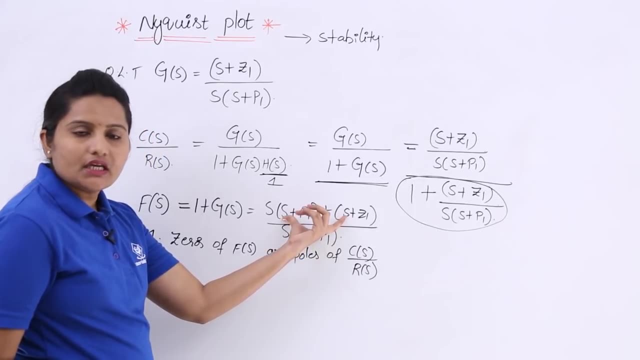 c of s by r of s, is it not? You can see zeros of f of s. that means these are zeros. the zeros of f of s are the poles of c of s by r of s, If you imagine this term here. 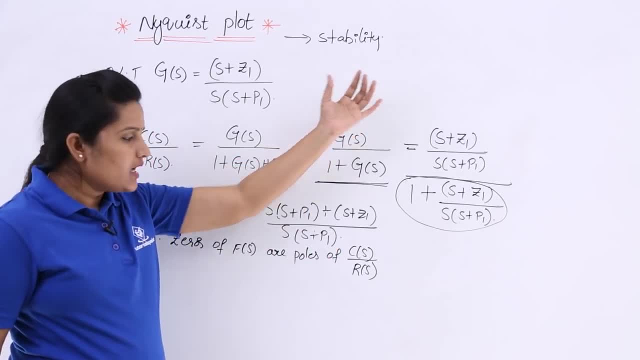 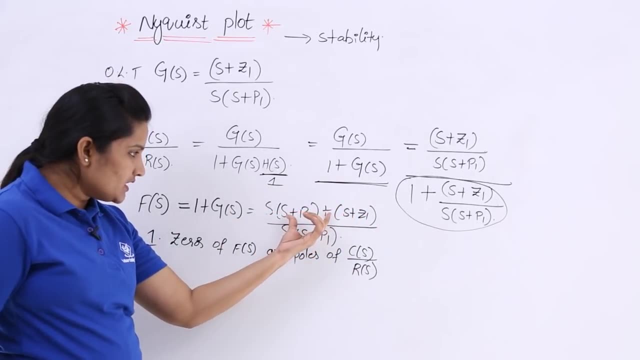 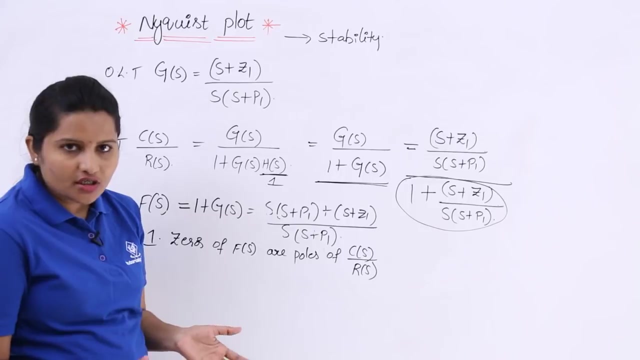 this denominator goes to numerator and here, whatever the value you are having in the denominator will be like this. So whatever the zeros of f of s, of F of S are there, those are mentioned as poles of C of S by R of S. In future, no need. 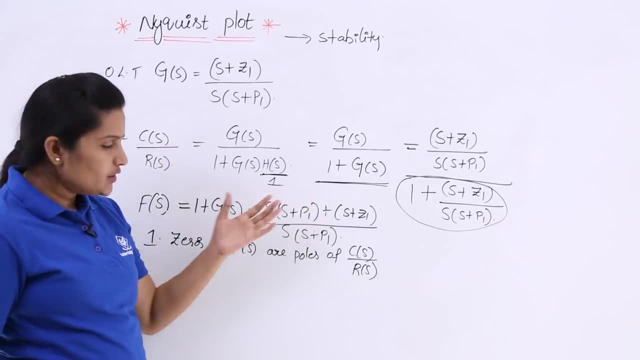 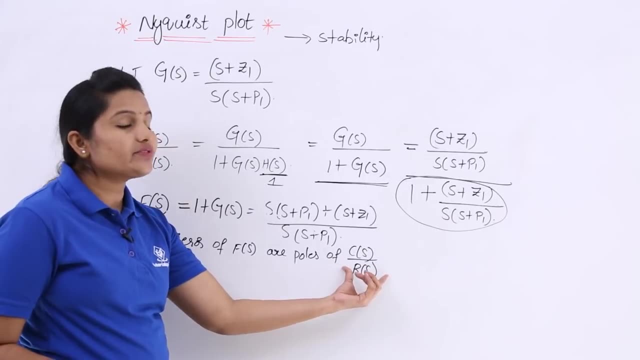 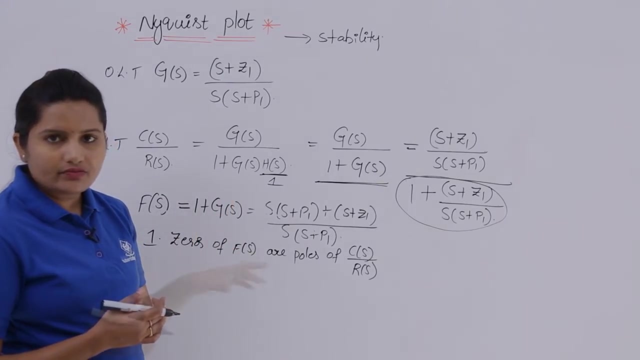 to calculate C of S by R of S for poles, you just consider 1 plus G of S. whatever is there in 0's place that can be considered as poles of C of S by R of S Coming to poles, poles of F of S. poles of F of S is equivalent to poles of G of S. For 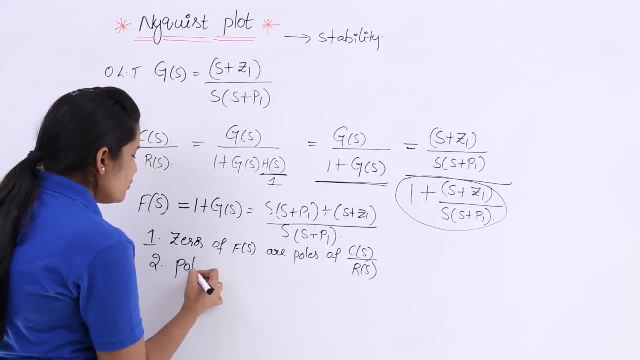 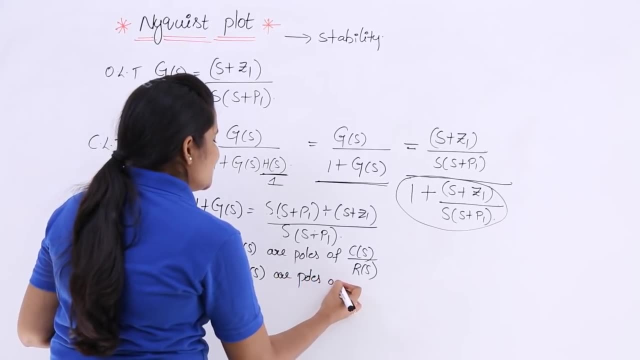 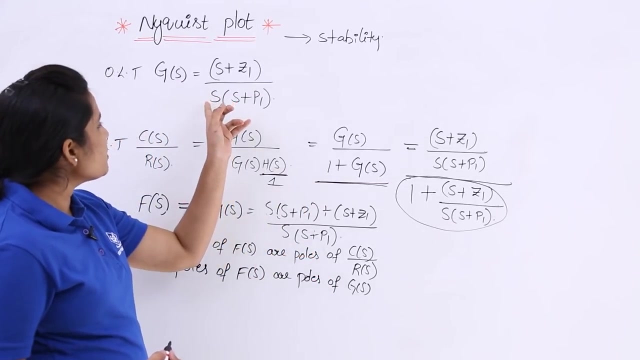 example. this second point you need to understand is: poles of F of S are poles of G of S. You can see, if you observe the poles of F of S, then if you observe poles of G of S, then these two things will be same. 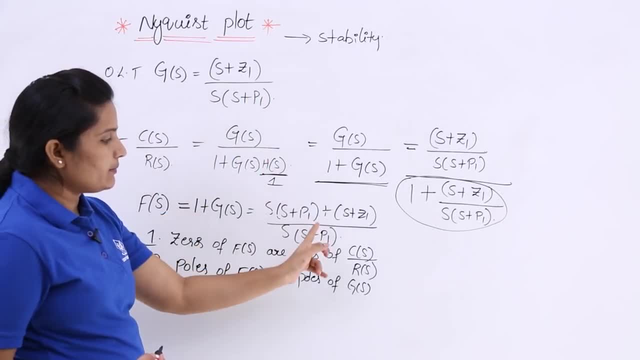 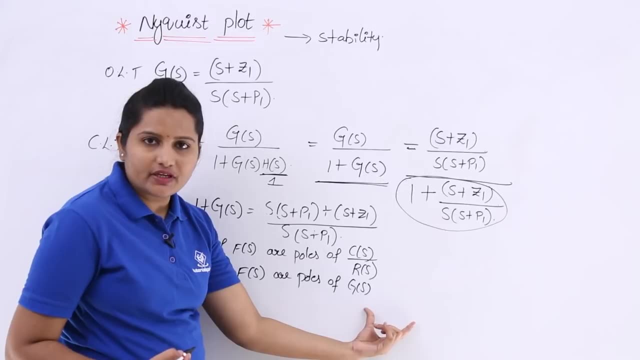 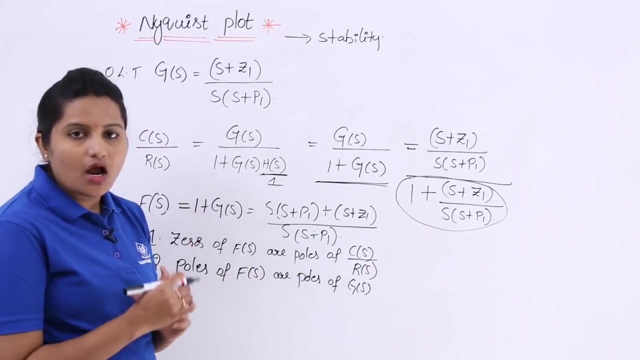 How does this come to be, How does this come to be of open loop transfer function? these two are same. So see here: poles of f of s are the poles of g of s and zeros of f of s are the poles of closed loop transfer function. c of s by r of s, whatever.